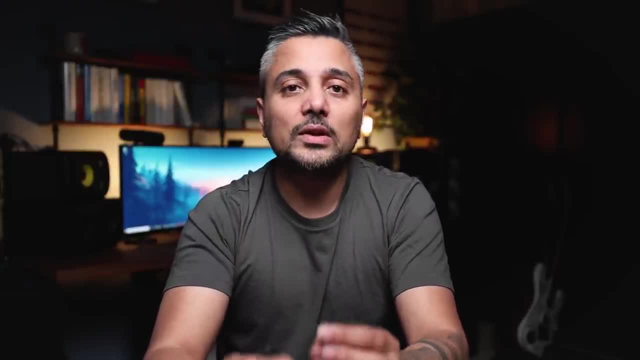 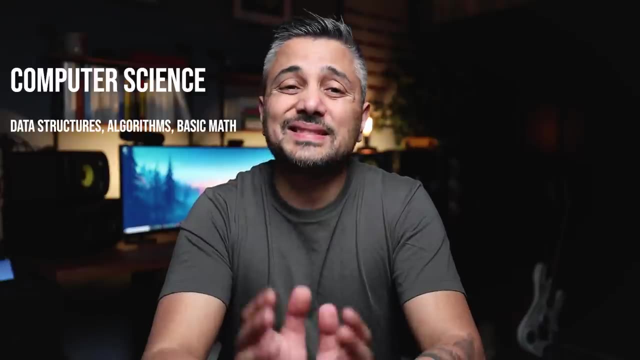 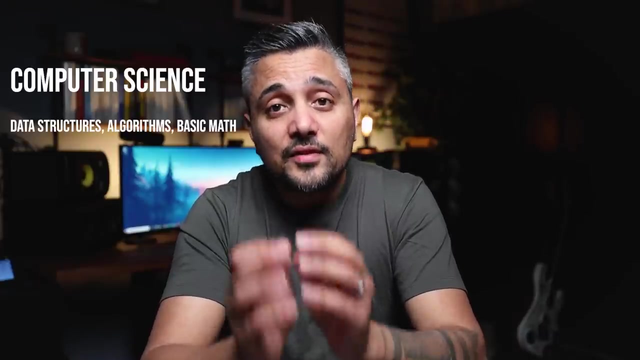 Ideally, both computer science and software engineering will cover the foundational computer science and mathematics knowledge. These are programming logic in one or more programming languages, data structures and algorithms, and basic probability, statistics and discrete math. And since computer science is a theoretical study of computers and computations, 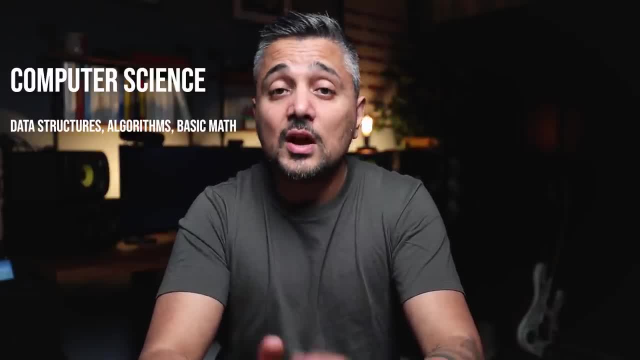 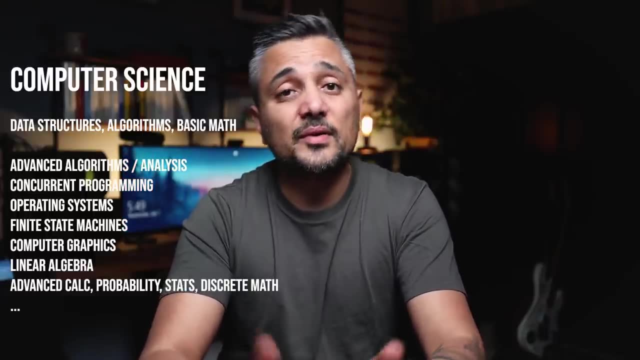 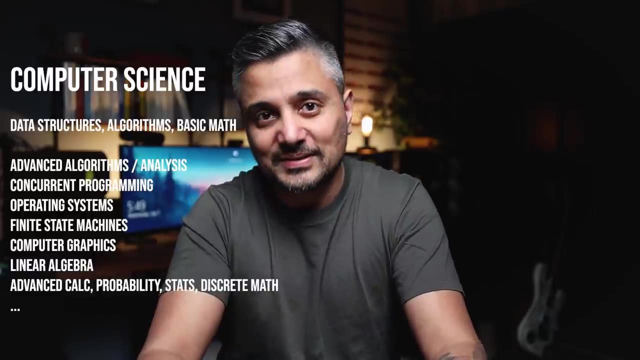 a computer science degree will build on that foundational knowledge with advanced topics in the same areas, For example advanced algorithms and analysis, concurrent programming, operating systems, linear algebra, advanced calculus, finite state machines and also other advanced mathematics courses. A computer 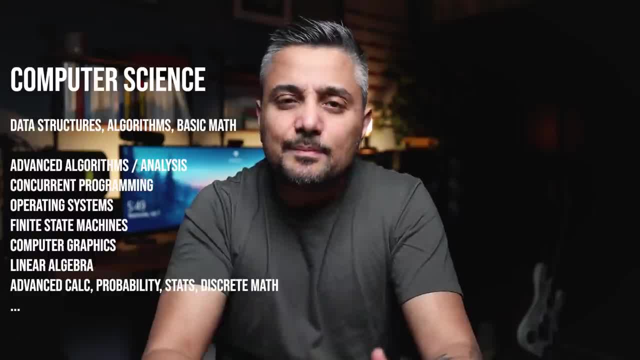 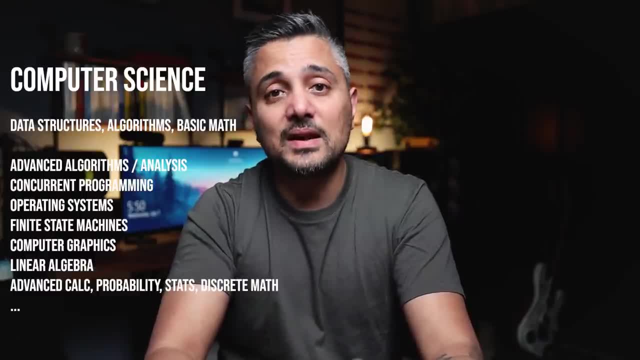 science degree is a great option for you if you love learning things at a very deep academic level. It is also a good choice if you plan on getting advanced degrees like masters or PhD in specialized areas like operating systems, distributed systems, data science, machine learning, so on and so forth. 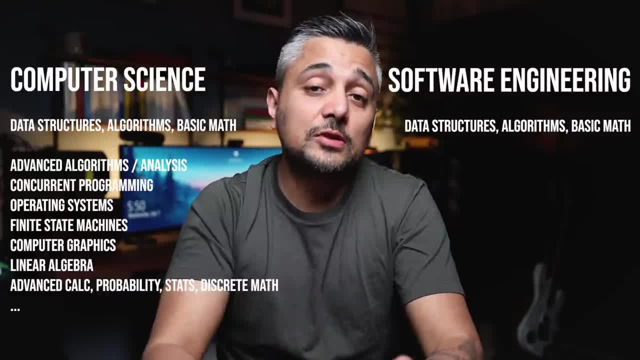 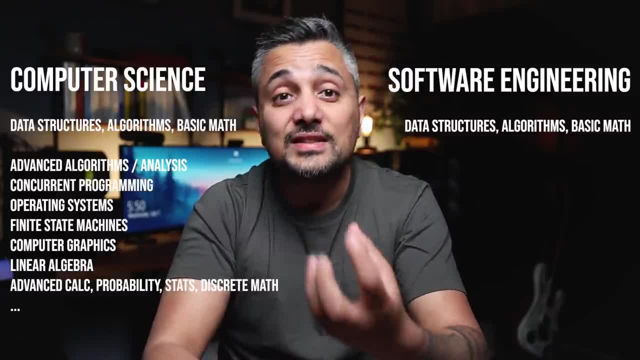 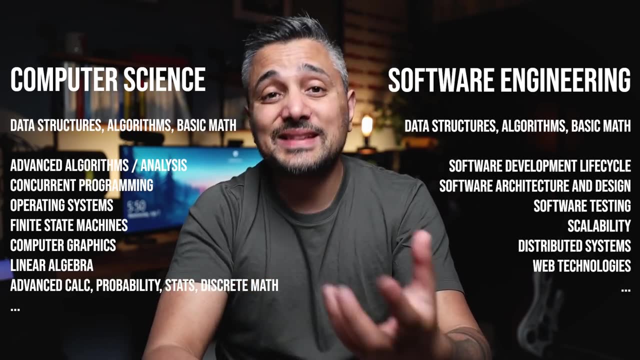 A software engineering degree will also cover the same foundational topics, But since software engineering is the application side of things, a software engineering degree will take the foundational knowledge and teach you how to build software systems that are used in the real world, For example, software development, life cycles, software design. that includes things. 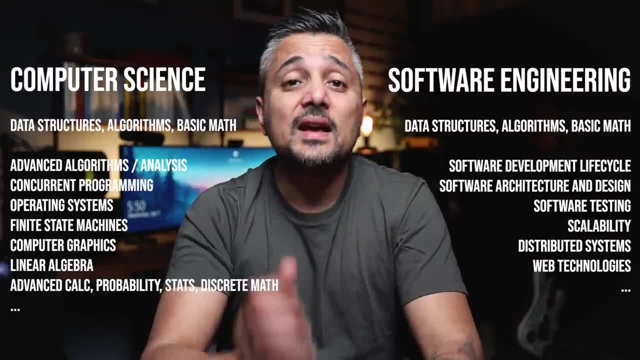 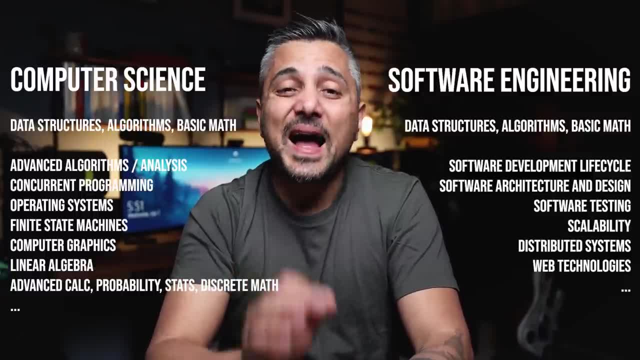 like design patterns, principles and paradigms, software testing, scalability, distributed systems and web technologies. A software engineering degree is a great option for you if you want to get a high level overview of engineering practices used in the real world, and also if you want to. 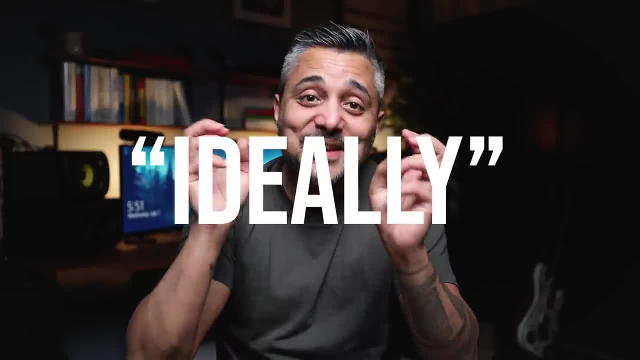 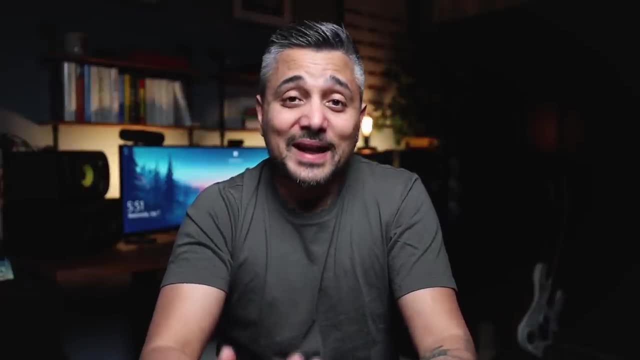 get in the industry right away. But notice that I said ideally when I started talking about these two degrees, because this is the by the book definition of what these degrees should be. But as with anything in the real world, it's not cut and dry Because there isn't a universal 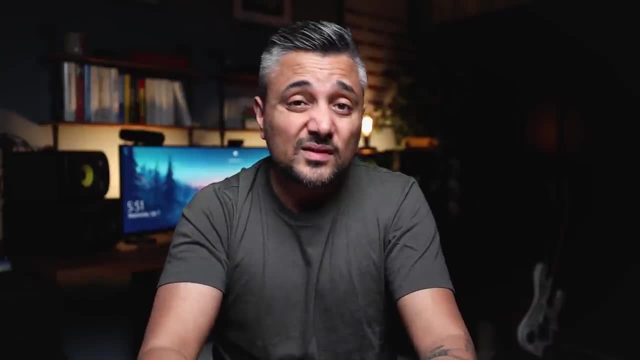 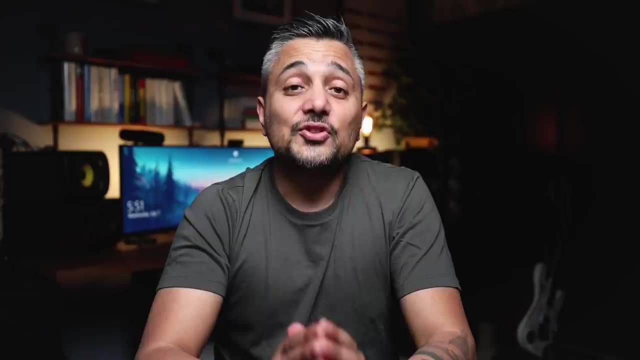 standard that regulates what these degrees should be and, as a result, these degrees can vary quite a lot from university to university, And, to that end, here is a few things that you need to watch out for. You need the fundamentals- Programming logic in at least one language. data structures. 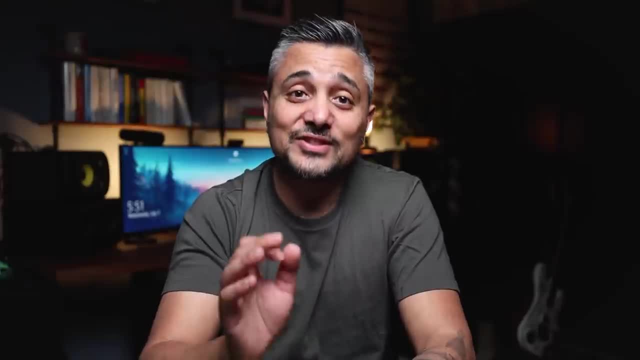 and algorithm. If a CS degree or a software engineering degree does not have that run the other way, Those aren't going to be good for your career as a software engineer or a developer. If you plan to do a software engineering degree in the real world, it's not going to be a good. 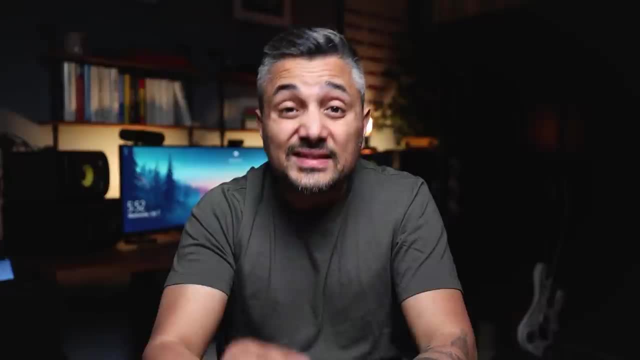 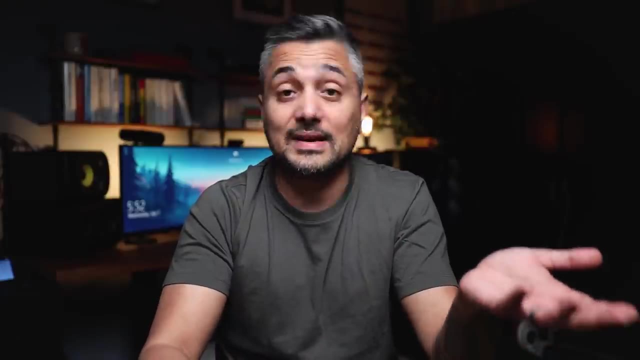 idea. If you plan to do advanced degrees in specialized topics, you probably want to go with a CS degree that has courses that cover a lot of theoretical knowledge and mathematical concepts related to the areas that you want to specialize in. This sets you up for success when 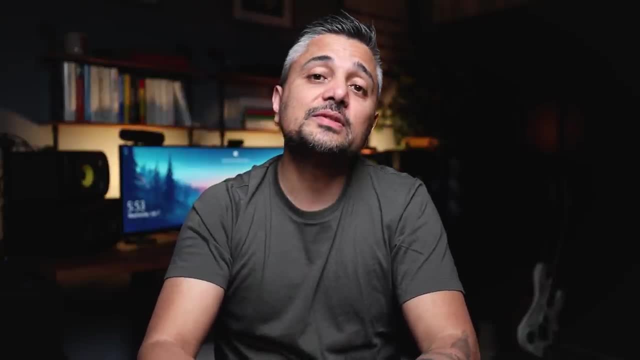 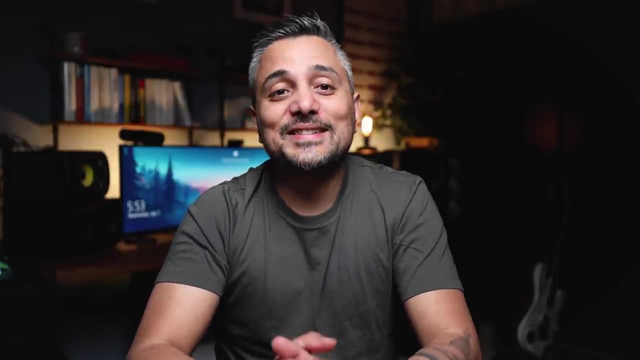 you pursue advanced degrees But at the same time, if you don't want to pursue advanced degrees, you probably don't want too much theory in your undergraduate degree. Not all software engineering degrees are made the same. Some lean heavily towards electrical engineering and physics. If that's what you want, that is cool. 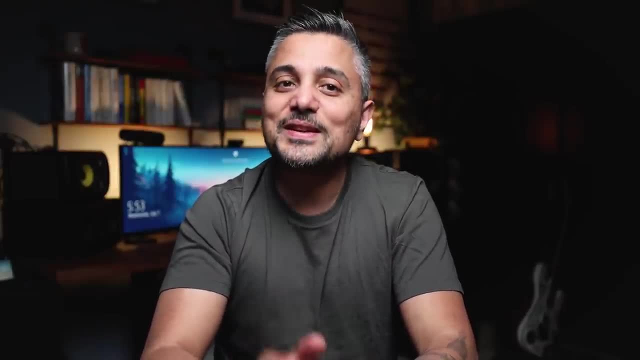 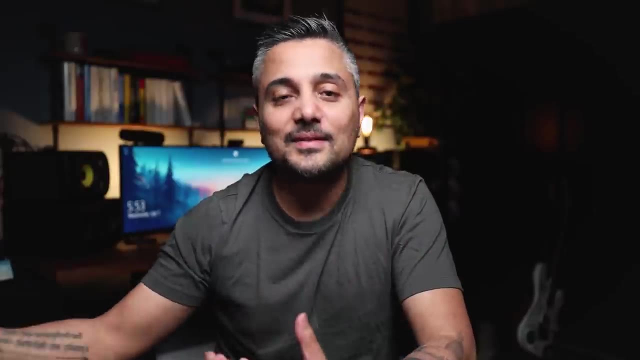 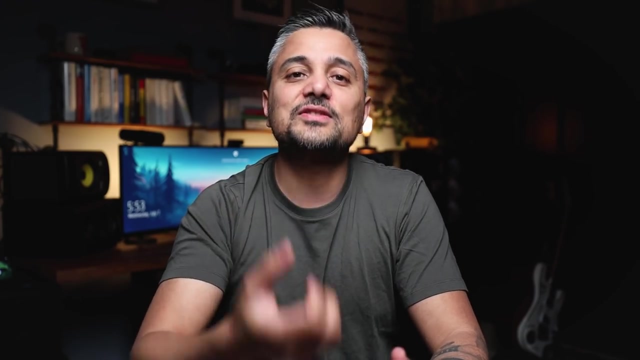 But if you want to stick to software engineering, watch out for too many classes in these areas. And then there are those degrees that linger around within the computer science and the engineering department, but they are neither engineering or computer science. They have their own merits, but they may not give you enough foundational knowledge or enough knowledge in 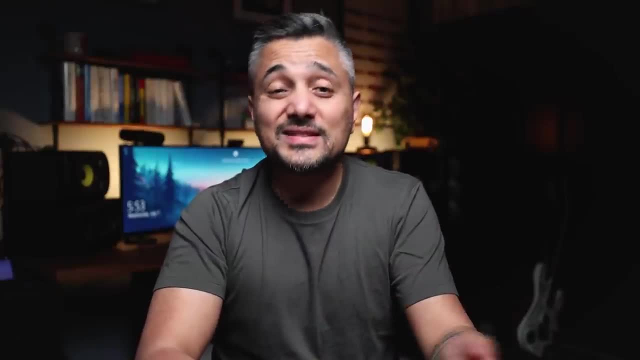 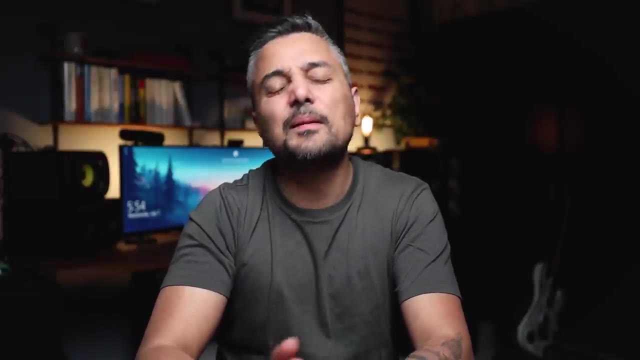 general to kickstart your career as a software engineer. These are degrees like information technology, information systems, data science, etc. They're fine as specializations, but I wouldn't recommend them as full degrees, at least not at an undergraduate level. 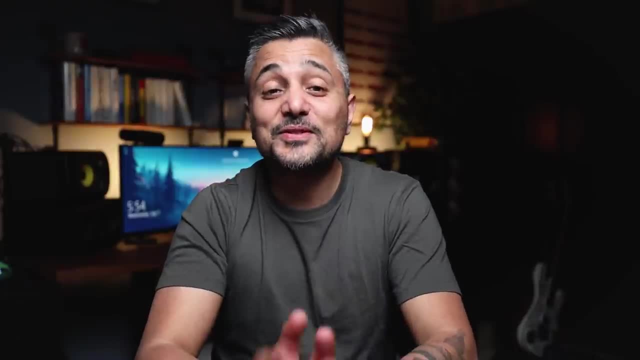 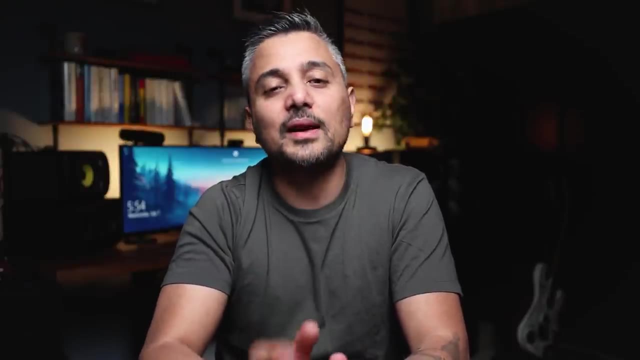 Okay, now that you know a few things to watch out for, let me give you some advice on how to go about picking your degree in general. See, the thing is that you need a bit of both theory and practical knowledge. Here's a real-world example. Say you're building a. 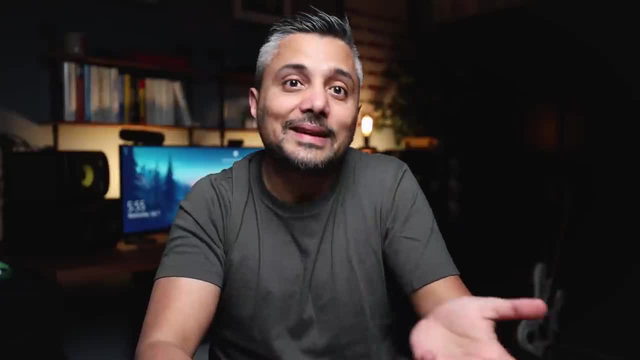 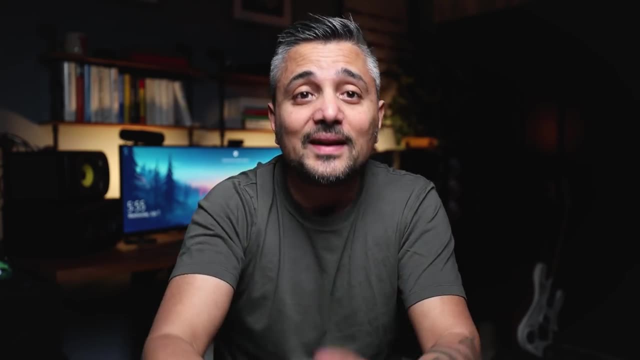 cloud-powered spelling checker like Grammarly or something like that. A computer scientist would likely think about what is the best way to find if a word is even misspelled, And from there, what is the most optimal way to find the best match for a suggestion. 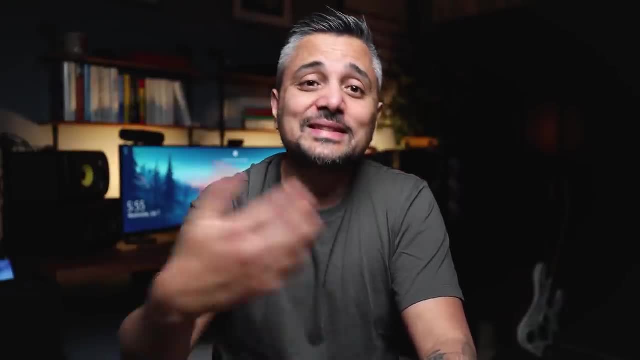 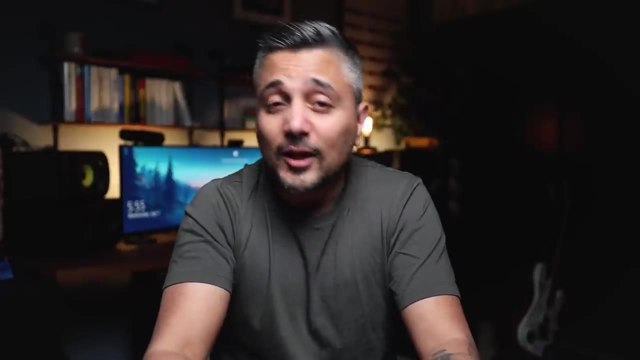 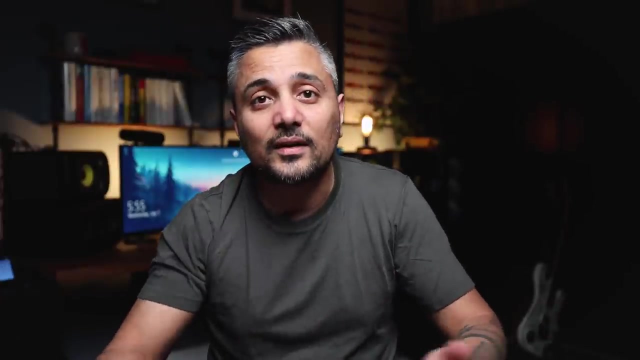 Could this be modeled as a graph problem where we find the Levenstein distance between the two words to find the closest suggestion? This is very theoretical and mathematical but it could help finding suggestions fast. But autocomplete is a part of a larger system like Grammarly or Microsoft Word. How would other parts connect to the system? Would the 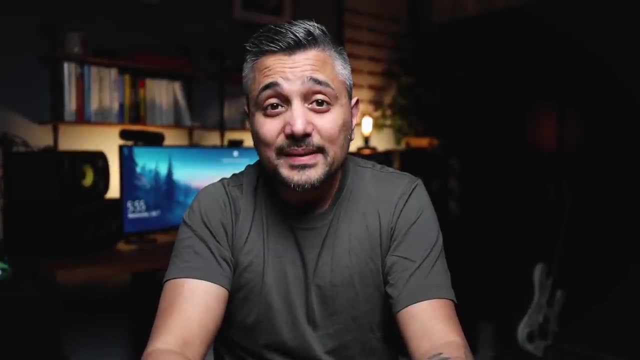 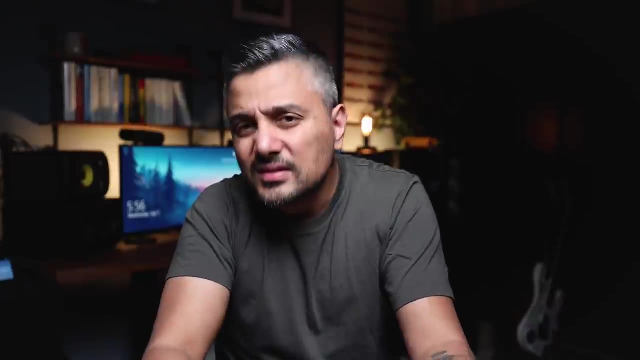 autocomplete, be exposed as an API? Would it be cloud-based? If so, what are they? Many of these things are hard to figure out in the dictionary. How do we observe the latencies and throughput? Should the dictionary remain in memory? How should we design the? 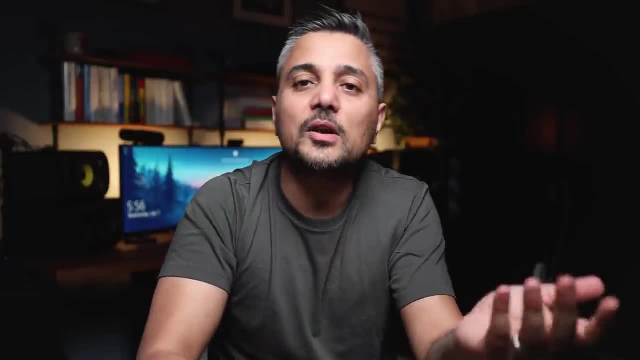 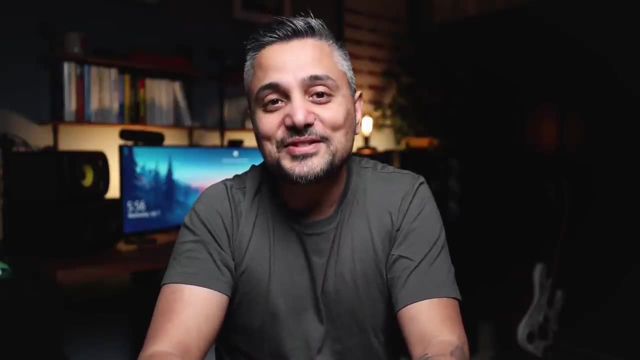 overall system. What if we want to completely swap out the current version of autocomplete with the new one? How would that affect other modules? How can we make a system extensible but decoupled at the same time? You get the idea. Remember our initial definition: Computer science. 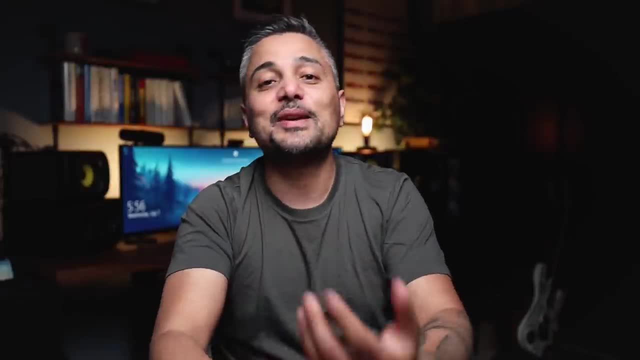 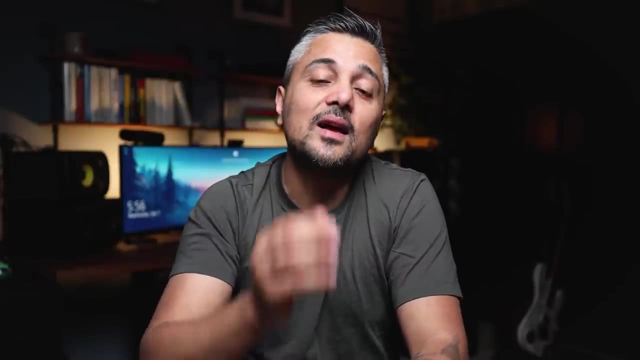 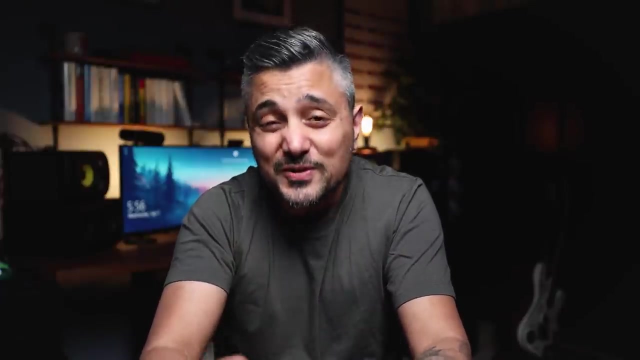 helps you understand how computers work or how computations are done In software engineering you to build software systems. so hopefully this real world example changes your perspective from obsessing about this degree versus that degree and instead thinking about how you can get the best out of your four years in college with a good mix of theory and practice. and for that here's my 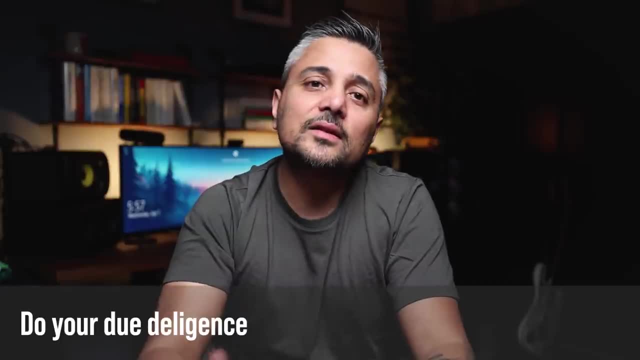 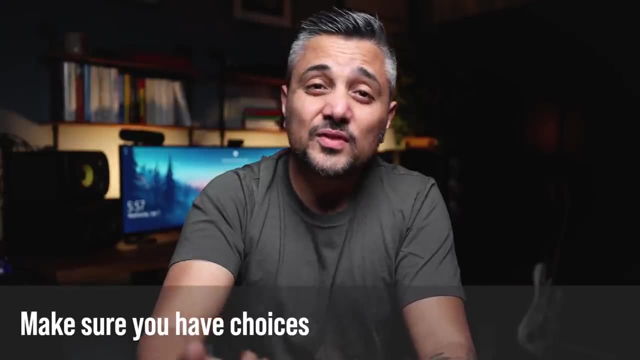 advice. first, do your due diligence. look at the curriculum to make sure that at least the fundamental courses are covered. second, does the degree give you choices to pivot on, or is it too structured and strict? is it too theoretical or too practical? ideally, you want a good balance. 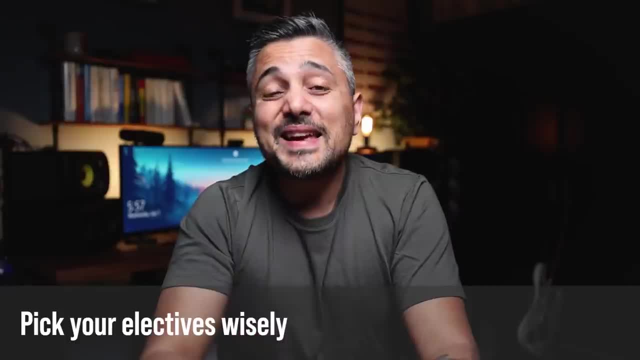 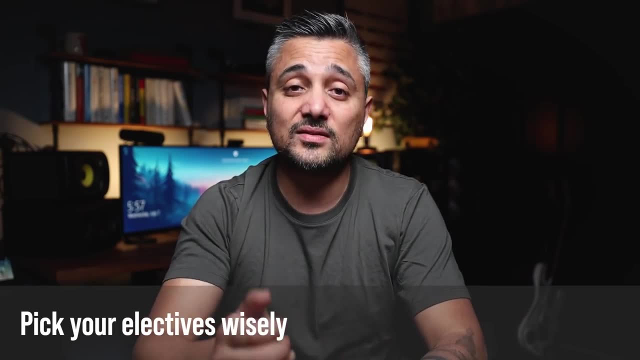 between theory and practice. three: think of a degree as a flexible canvas. you should have the option to choose from a wide variety of electives to shape your degree however you want, based on your own interest or the job market. good programs give you this choice. the only thing that 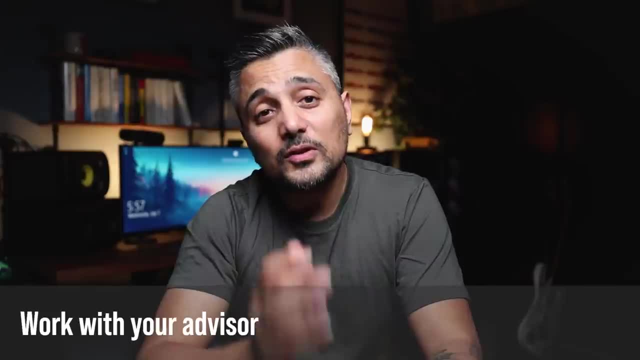 should be forced upon you are the fundamentals. fourth, work closely with your advisor and let them know what your goals are to create a course plan that fits your need. and find out what your goals are and what you need to do in order to achieve your goals. and find out what your goals are and find out what your goals are. and find out what your goals are. and. 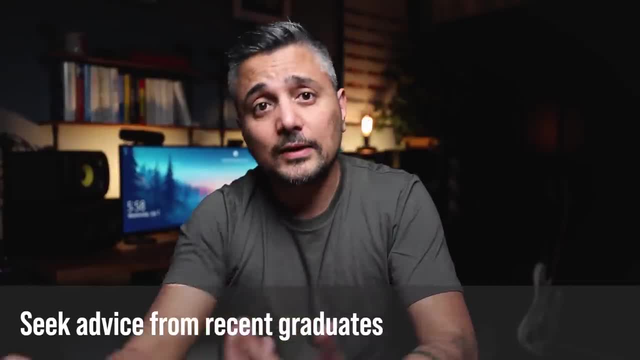 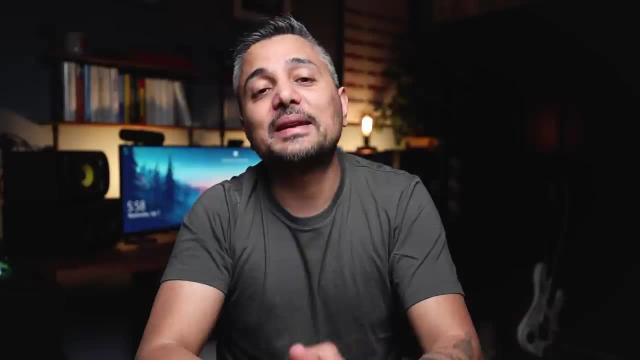 finally reach out to recent graduates, who you know that have recently gotten jobs, ask them about what classes they took and what helped them in their jobs. well, hopefully this gives you some idea on how to go about picking a degree but, more importantly, how to think about your degree, not as 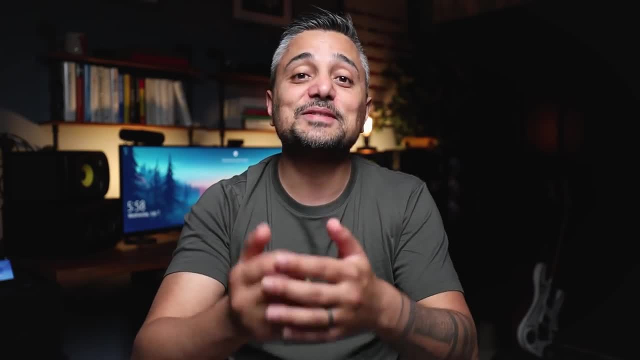 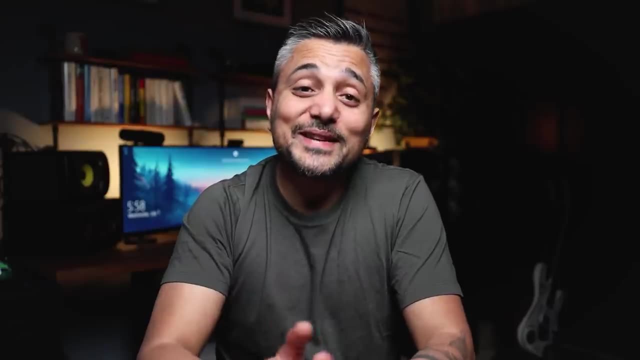 a computer science versus software engineering debate, but as a four-year stretch of learning that you want to get the most out of learning is the most important part in this debate. if you have sorted that part out, arguably you don't even need a degree at all. people without degrees have gone on. 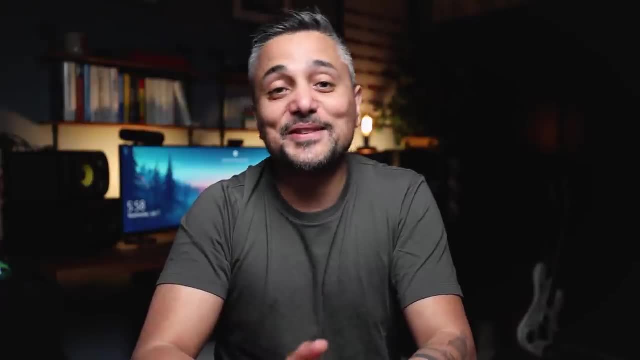 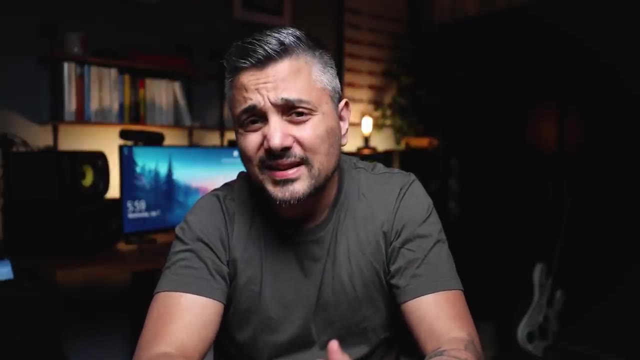 to build amazing software. well, i think i'll start venturing out into philosophy if i continue any further, so i'll stop here. let me know in the comments below what degree you have- computer science, software engineering, some other degree or no degree at all- and i'm also curious to know how.